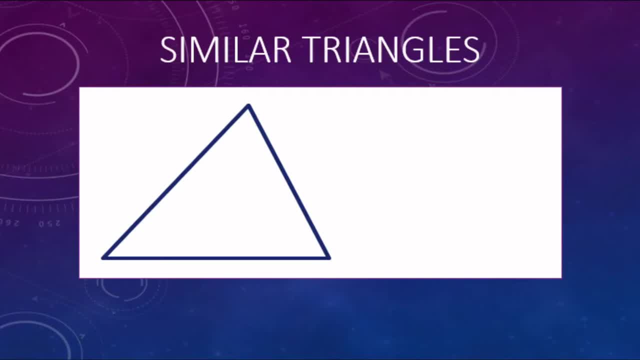 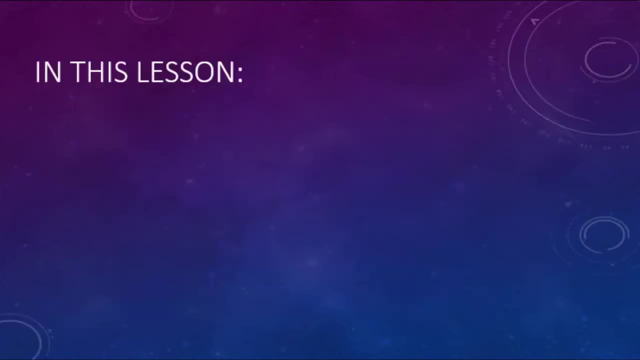 All right. so in this video we are going to be looking at similar triangles. Now, similar triangles come from a dilation. Now, when we have dilated triangles or polygons, all the corresponding angles are congruent, In other words, they're equal in measure and also the sides are proportional. So that's what we're going to be looking at in this video. here We'll be looking at the angles of similar triangles and we'll be using proportions to find missing side lengths in triangles. It's indirect measurement. 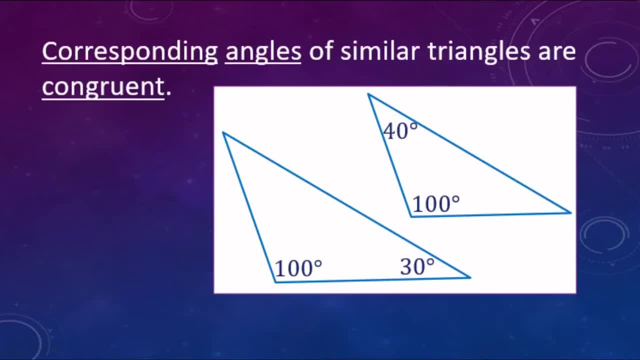 All right. so if we have similar triangles and we know that the corresponding angles are congruent, In other words, they have equal measures for the angle. So basically, what we're trying to do is match up the angles of the triangle. So like, let's look at this angle right here, It's corresponding angle is 40 degrees. So if it's 40 degrees on this triangle, then it's going to be 40 degrees on that triangle because they're corresponding angles. Likewise, if we're looking over here, that's going to be. 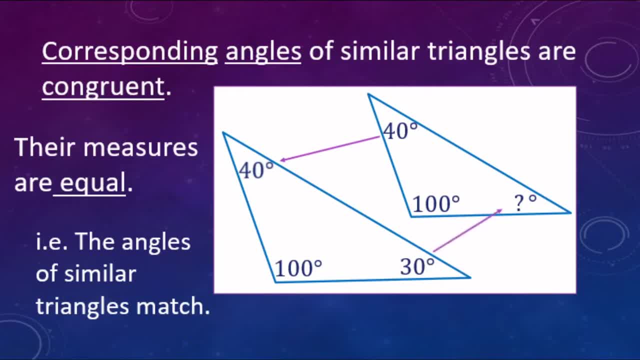 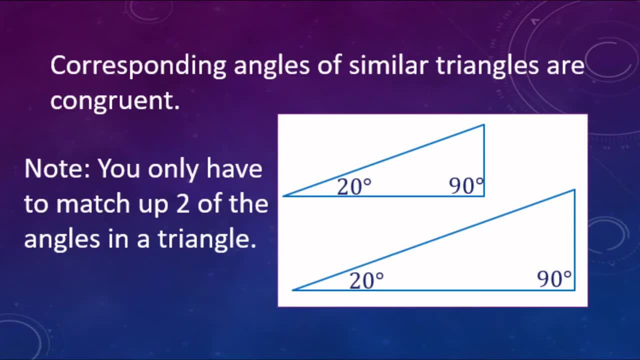 corresponding with this angle. So if this one's 30, then that one over there is 30 degrees as well. Now, to see if triangles are similar, you only need to match up two of the three angles, because- check it out here- In order to find this third angle up here, we need to start with 180, because we- all three angles- add to 180 and then we're going to subtract off the 20 degrees and also subtract off the 90 degrees, So that's going to make this angle 70 degrees. So if we know two, then we can find. 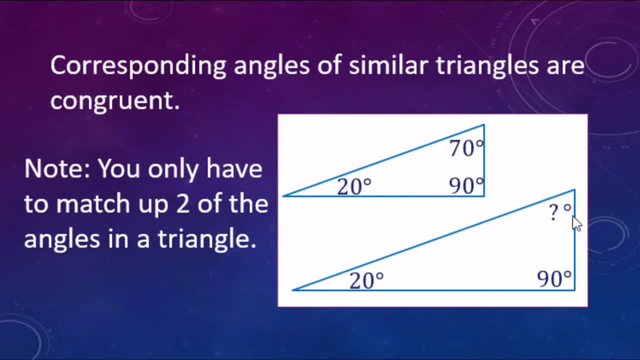 third one. now check it out with this other one. start with 180 to find this angle here. and you're doing the same thing: 180 minus 20 minus 90 equals again 70. so now we have all the corresponding angles are congruent where we only needed two, because in triangles, if you know two, you 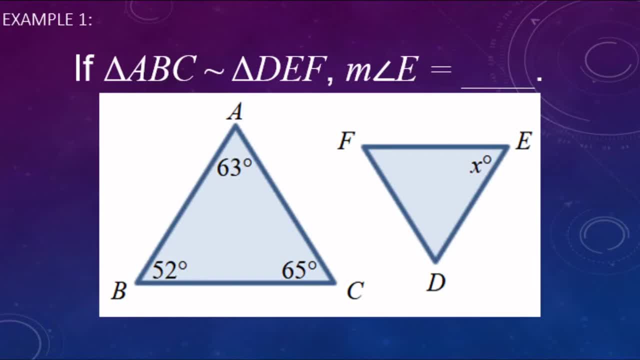 automatically know the third one. all right, let's look at this example here. so now these two triangles are similar: triangle abc similar to triangle def. this symbol does mean similar. now these two triangles have been like flipped and rotated and all that stuff, so they don't match. 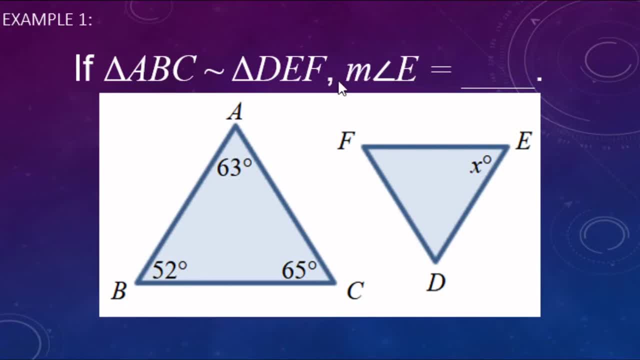 up perfectly like the last ones. so we have to use the notation up here. so if you look here the a and the d are in the first position. so that means vertex a and vertex d are corresponding vertices or corresponding angles, in this case here the middle ones, that's the b and the e. so that means 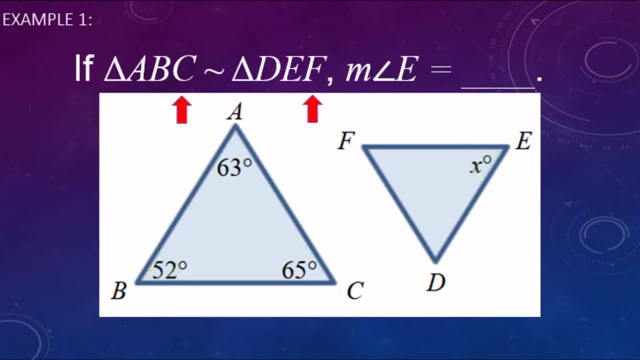 that b and e are the corresponding vertices. and then looking at the lasts, c and f, there's c and f and right and left and right and left and right and right and left and right and left and right and red. so again, when they've been flipped and rotated and stuff, you have to use the notation up here. 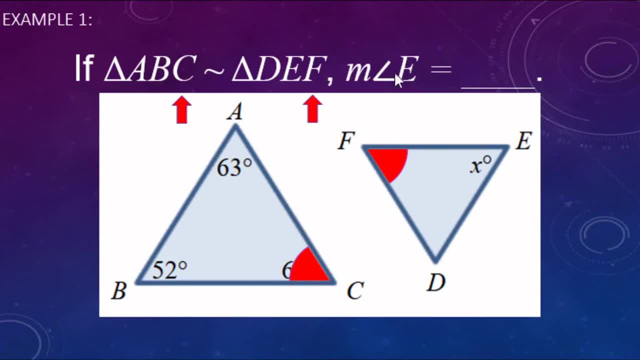 because they don't match up just by the picture. so here we're trying to find the measure of angle e. so angle e, right here marked with an x, it's in green. so remember e was in the middle and b is in the middle. so that means those two vertices match up. so if b is 52, e is 52 because they are. 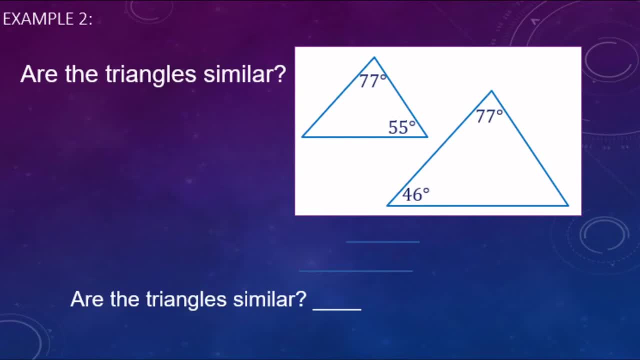 corresponding angles. all right, so are these two triangles similar? so basically, what this question is: are the corresponding angles congruent? so do our angles match up? it's kind of what we're thinking here. so let's just look at this angle right here in the corner. i got it in yellow. 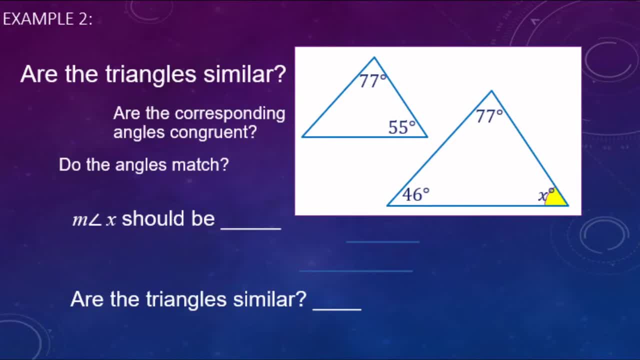 so x should be. so if these two triangles are congruent, its corresponding angle would be here. these two are corresponding, so x should match. it should have a congruent angle measure. so x should be 55 degrees. so now let's actually calculate the measure of angle x. so again with: 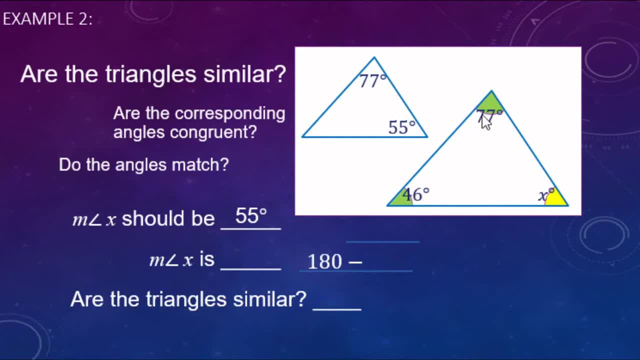 the interior angles of a triangle, they add to 180. so we're going to subtract the two other angles, the green angles, from 180. so the 77 plus the 46 makes 123.. now, of course, you could do it like what we did on the last example there, where we just subtract 180 minus the other two, looking like this: 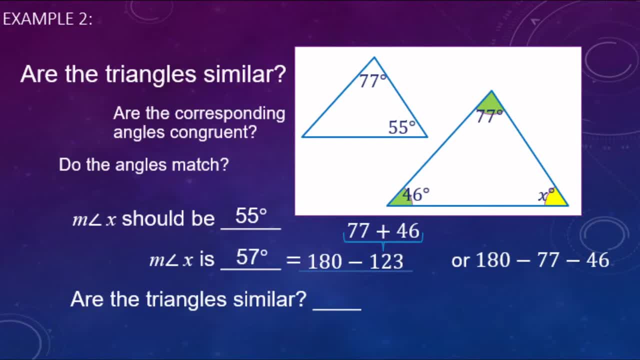 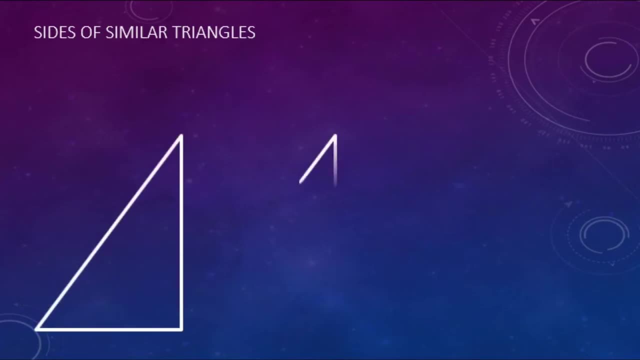 either way, x actually equals 57 degrees. so are these two triangles similar? no, if they were, x would be 55 degrees, but instead it's 57 degrees. so now let's look at sides of similar triangles. so here's three similar triangles up on the screen. 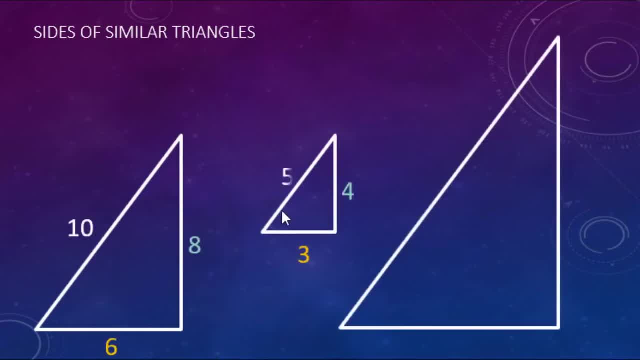 side lengths of the one on the left, six, eight and ten. we got three, four and five for the middle one and the big one nine, twelve and fifteen. so we're going to be looking at the ratio of side lengths. so we're just going to be using right away just the, the green and the orange one. 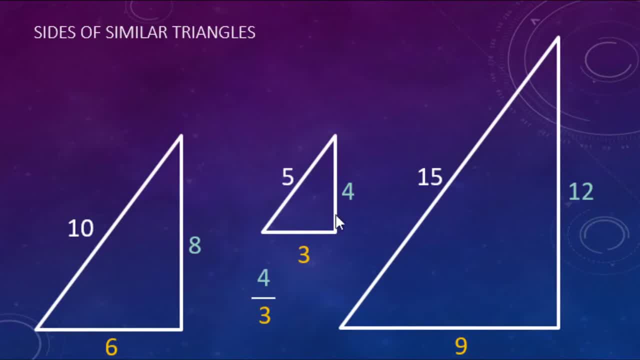 so that's going to be a four, two, three ratio for these two sides here. looking at the same two sides again, we're looking at corresponding sides as being eight to six ratio, which is the same. it's, uh, reduces to four thirds, and then for the big one, that's going to be a 12 to 9 ratio, which also 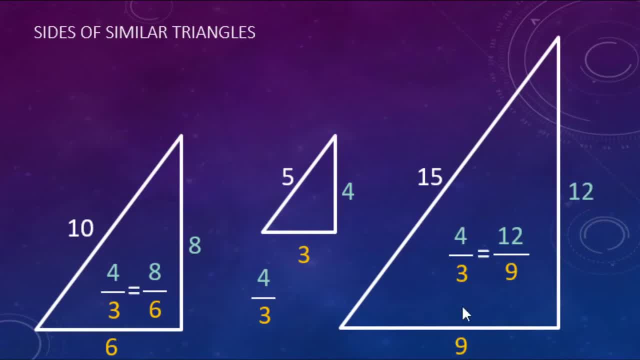 reduces to four thirds. so the pairs of sides here all reduced to four thirds so that we have equal ratios. so in other words, the side lengths are proportional and this works even on the other sides, like five to three is the same as fifteen to nine. they both reduce to the same thing. 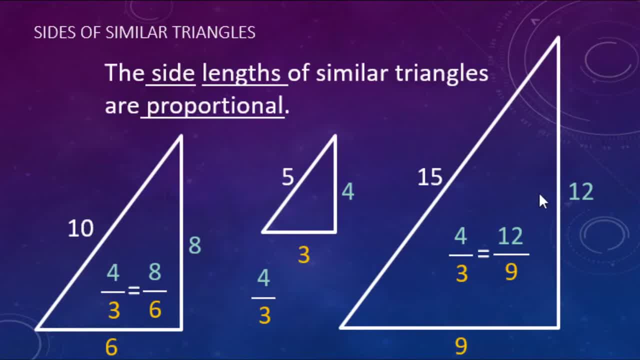 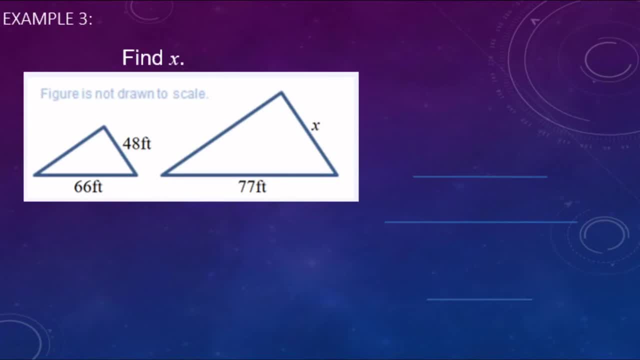 ten to six, or you can go ten to eight, five to four and fifteen to twelve. all the pairs of sides are proportional. all right, for this example, we are going to be finding this missing measure here, this x, right there. so since these triangles are proportional, they're similar. so the sides. 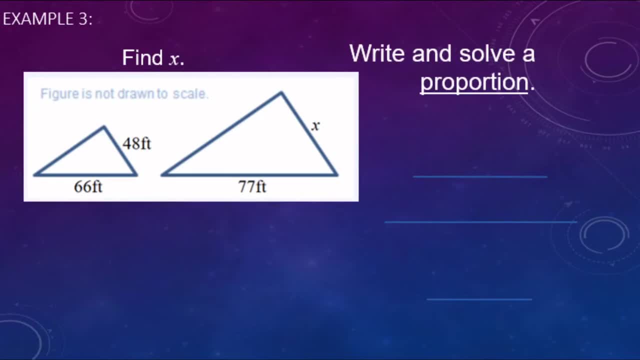 are proportional. we're going to write and solve a proportion. now, proportion is two equal ratios. so we got a ratio here equals another ratio here. so this ratio on the left, we're going to do with the triangle that's on the left. so we're going to use the 48 and the 66 because they 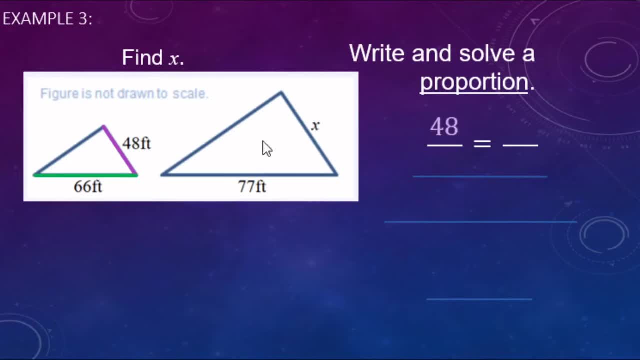 correspond with the x and the 77. so here we go: 48 for the numerator and then 66 for the denominator there. so there's our ratio on the left side for the triangle that's on the left. now the ratio that's on the right, we're going to use the triangle that's on the right. so the side lengths. 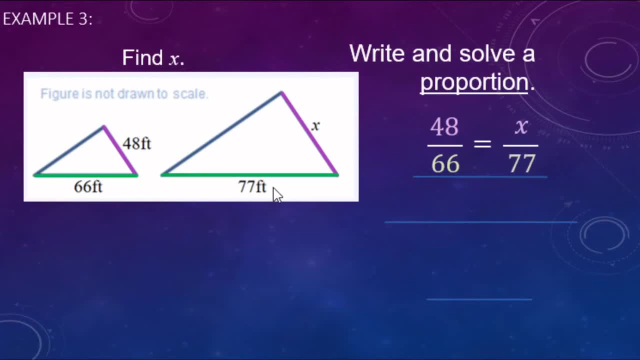 x, which is what we're trying to find, and then 77. so there are four different correct proportions that you can set up. this is just one of those four, and then for solving these, there are different ways. you can treat it like an equation and undo. 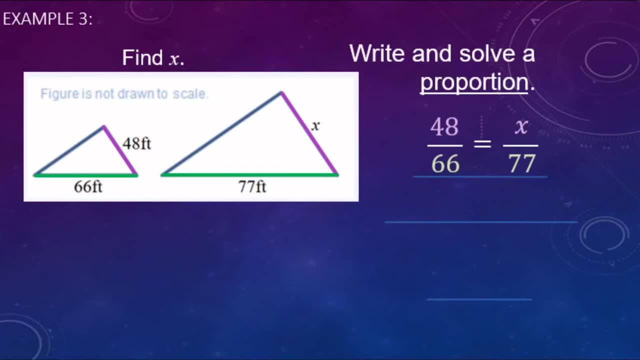 operations. but for this one here we're going to do cross multiply. so here we go. we want to figure out what x equals, so we're using cross multiplication. so we're going to do 48 times 77 cross multiply there, and then for the other diagonal, 66 and times x. 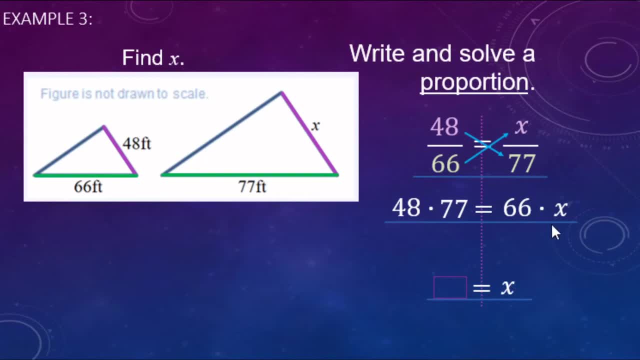 so again we're trying to get x by itself here. we want to undo the times 66 to the x, so we're going to go back down and we're going on by sorted inside and then we're going to do cross multiply and that's going to be one half. so we're not going to do cross multiply of x, but we're going. 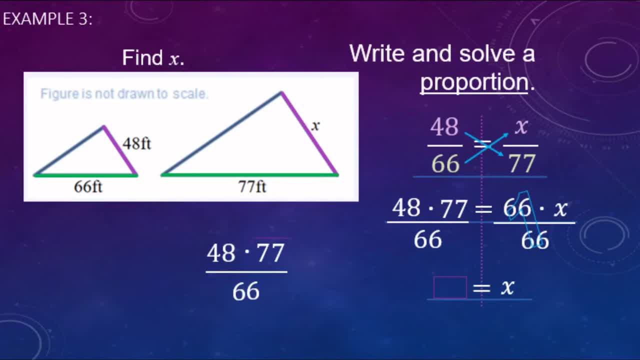 to do cross multiply of x. so i want to do this alphabetically. so we start with 66, and how many are there that we can do cross multiply? we from theufen of x- we're going to grad that as well- and from that, and we're going to do the both times, Dash to the x, and that will give us this: and so we're going to do the both times Dash to the x, and that's going to give us a cross multiply of x and to the X of x. that will make this our solution. and if we want to do more cross multiply, well, that would be if we, where we would be doing this with saying vec Ala, purchasing or removing of common factors. 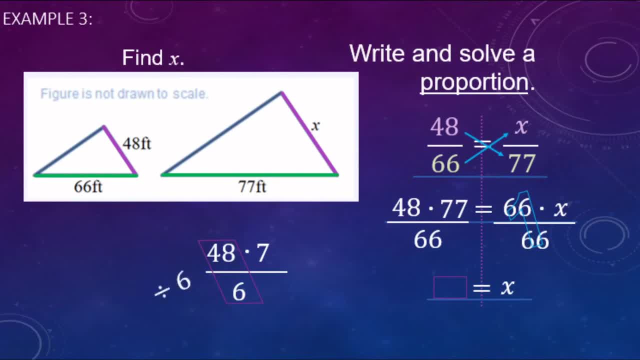 So in this case here the 48 and the 6, they're both multiples of 6.. So we'll remove a factor of 6 from both the numerator and denominator, And again we're thinking division with that, And so we end up with 8 times 7, which makes 56. 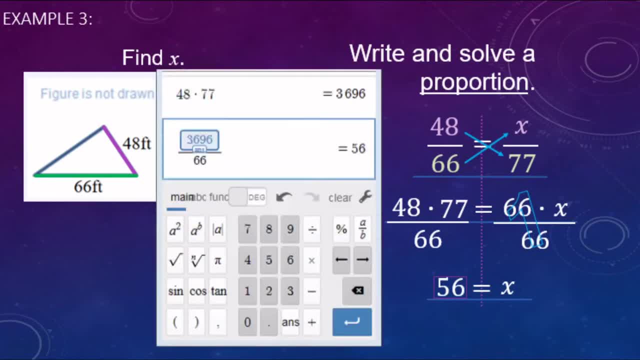 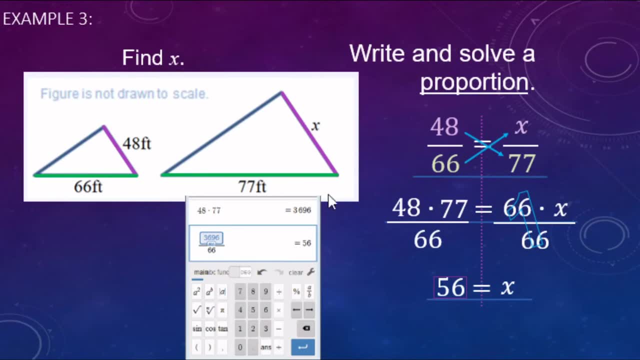 Now it is okay. if you want to go ahead and use a calculator, You can totally do that. I got that shown on the screen as well. So there you go, Solving using a proportion for a missing side length of similar triangles. 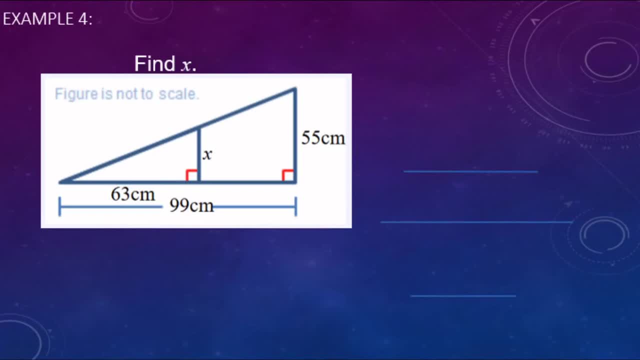 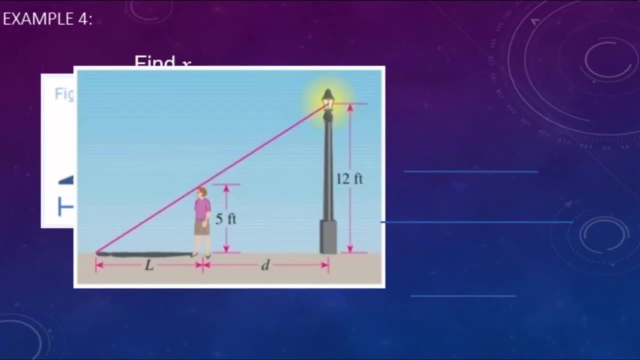 All right for this example. here we are going to be finding the measure of this length here. Sometimes we'll see triangles similar to what's going on, Like if you have something really tall and then something smaller and there's some sort of shadow involved and you end up with a big triangle. 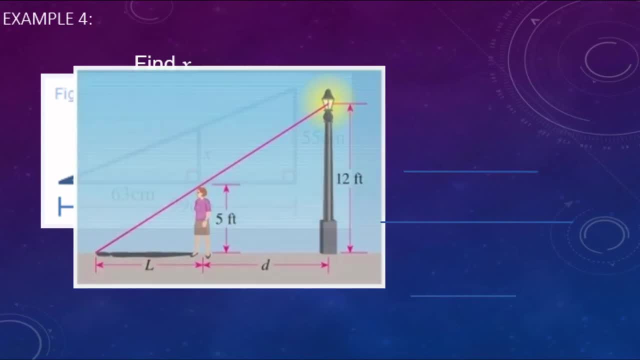 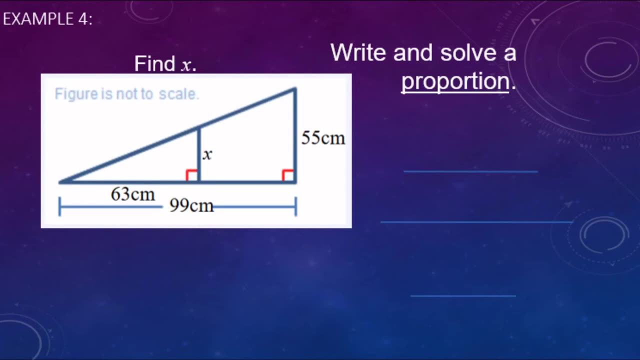 and then a smaller triangle there, which are similar. So that's what we're going to be doing here: We're going to be finding the value of this length here, which is where that person was standing, And so we are going to do, write and solve a proportion. 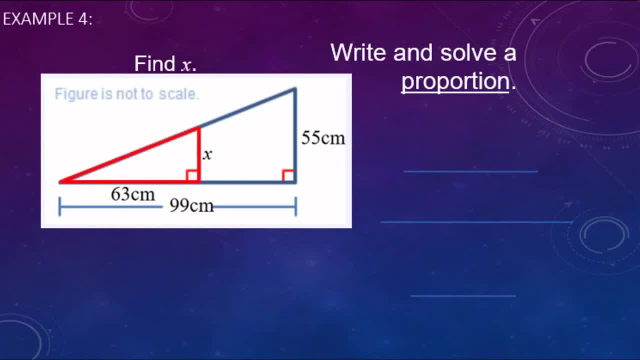 Now, when you do that, you're going to be finding the value of this length here. and when you have overlapping triangles, sometimes it is a good idea to go ahead and redraw it, so that way the two triangles are not overlapping anymore. 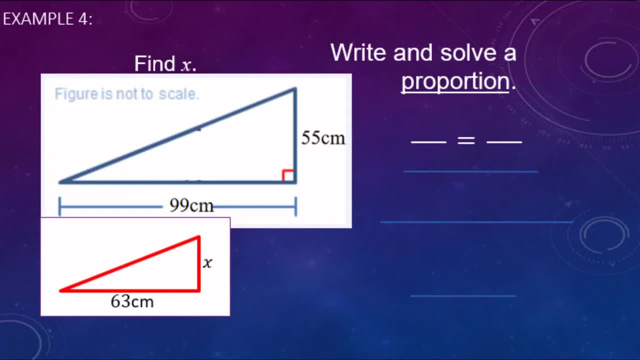 So we can redraw the small one off to the side. And now we're ready to write out our two equal ratios. So this first ratio it'll go with the small triangle, so the triangle that was red there. So X for the vertical side and then 63 for the green, the horizontal side. 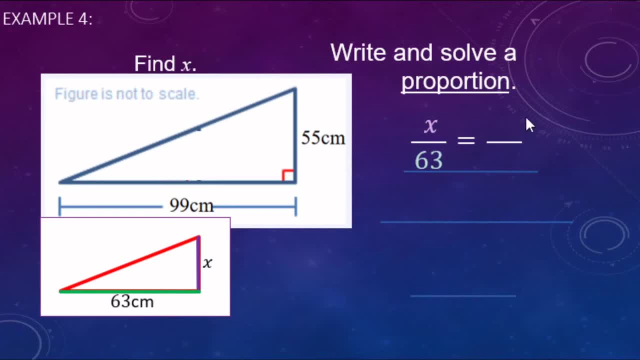 So there's our first ratio with the small triangle, And then our other ratio will go with the big triangle here. So the two sides that we'll use is the 55 and the 99.. So 55 over and then 99.. 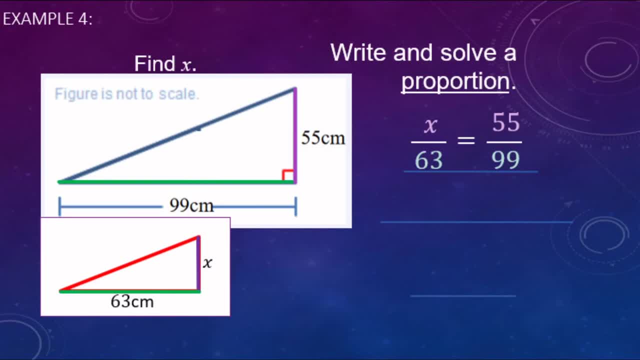 And now it's similar to the last example. We're just going to solve using cross multiplication. So we want to figure out the value for X, So we're going to do cross multiply, So we're doing X times 99 for that first diagonal that we're multiplying. 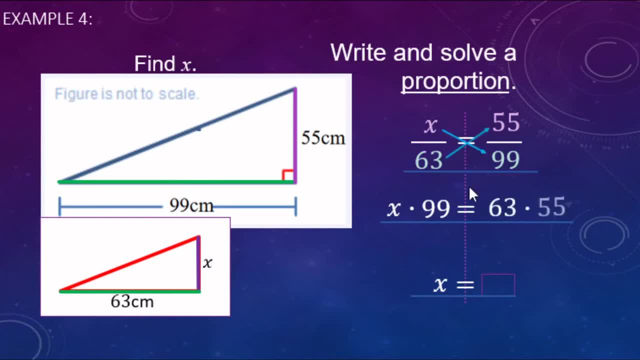 And then the second diagonal is going to be 63 times 55. Now we do want to get rid of that. We're going to get X by itself, so we have X times 99. We just want regular X. We're going to undo that times 99 with a divide by 99..